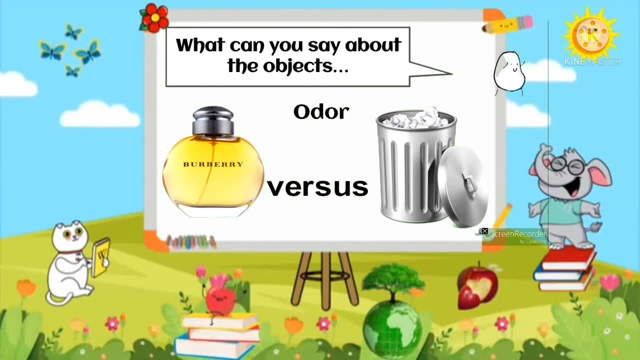 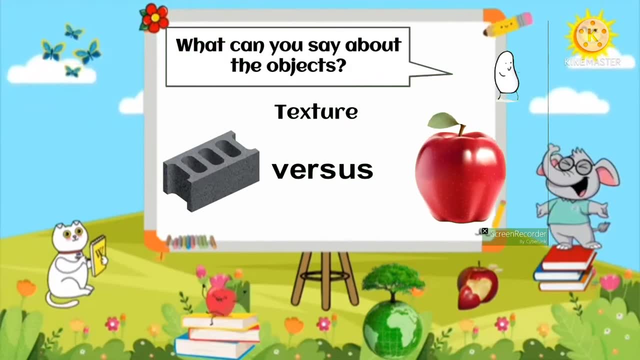 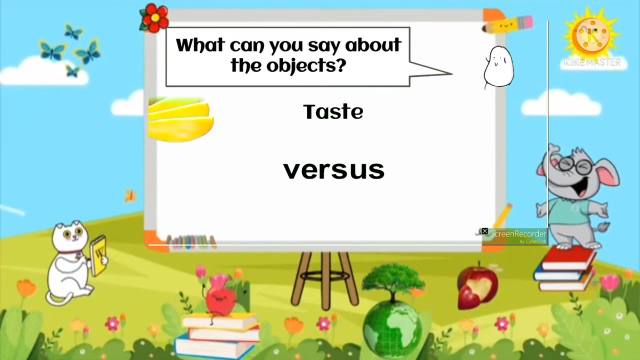 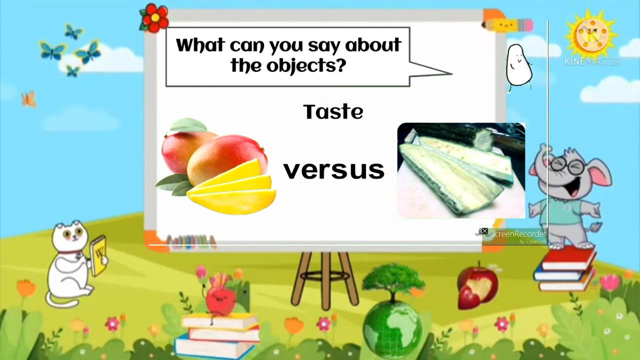 We compare their odor. What can you say about the object's texture? Yes, you're correct, The hollow black is rough while the apple is smooth. We compared their textures. What can you say about the object's taste? Alright, mango is sour while ampalea is bitter. 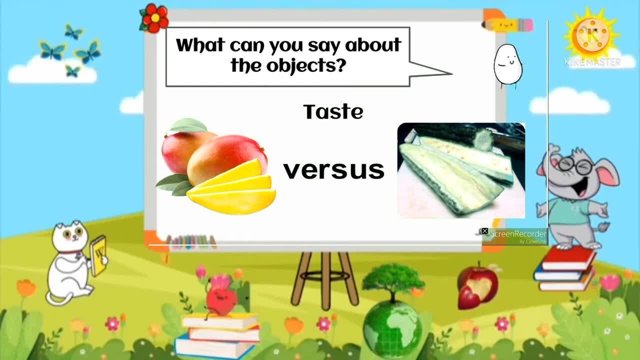 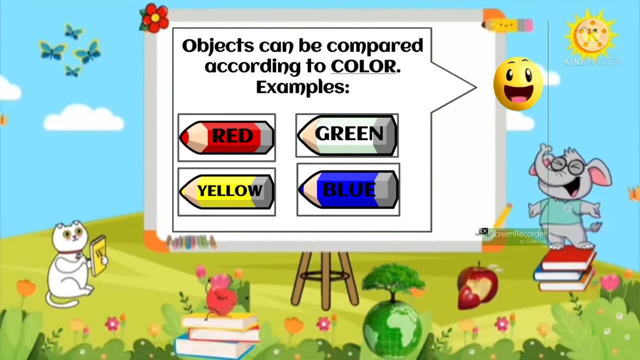 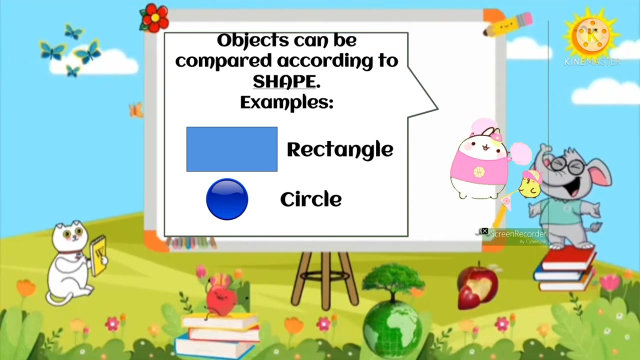 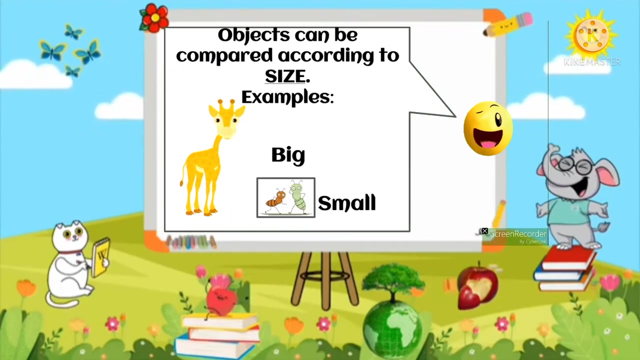 We compared their taste. Objects can be compared according to color: Examples: red, yellow, green and blue. Objects can be compared according to shapes: Examples: rectangle and circle. Objects can be compared according to size: Examples: big and small. 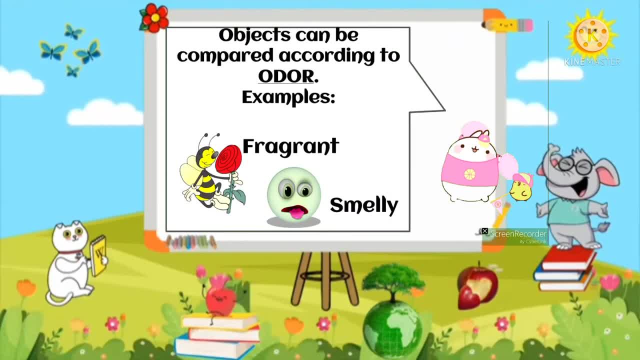 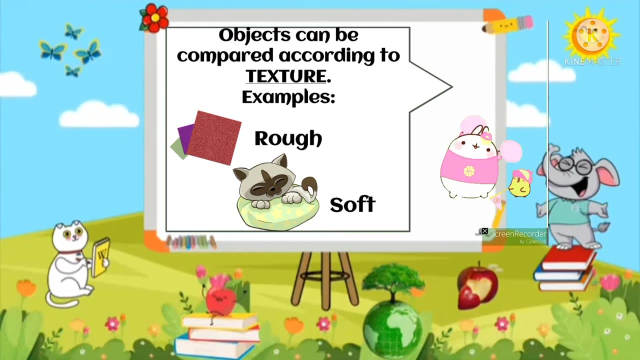 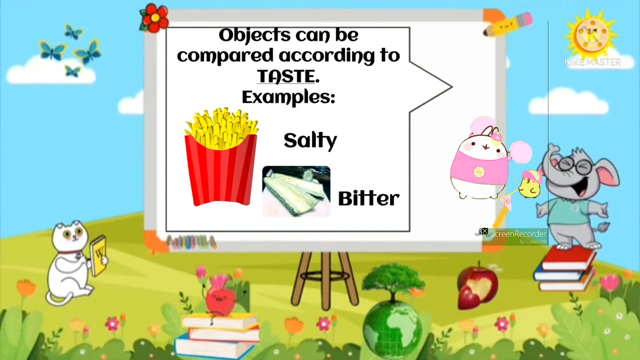 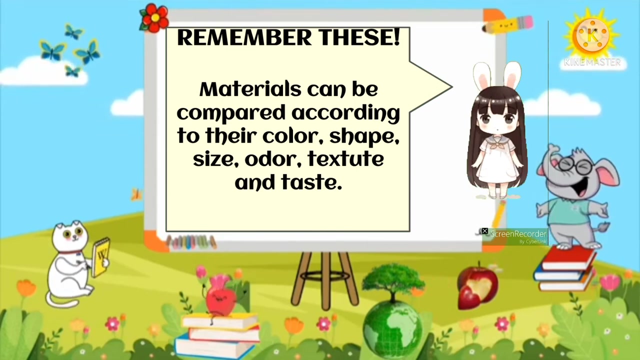 Objects can be compared according to odor: Examples: fragrant, smelly Objects can be compared according to texture Examples: smelly, Rough, soft Objects can be compared according to taste Examples: salty, bitter. Remember this: Objects can be compared according to their color, shape, size, odor, texture and taste.